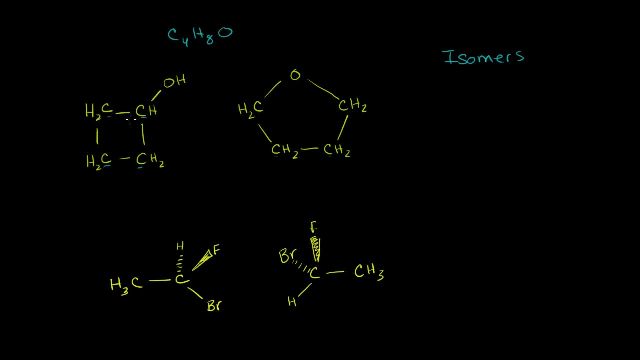 and they're a special type of isomer. In this situation, we don't have the same bonds. We're made up of the same things, but the bonds what is connected to what is different. So we call this a constitutional isomer. 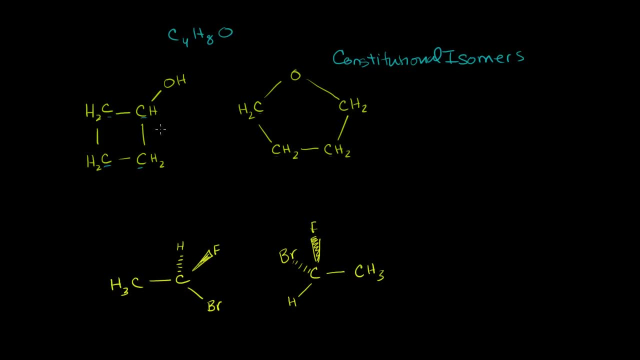 So we are essentially made up of the same things, but we are actually two different molecules, actually two very different molecules here. Now let's look at this next guy over here. So if we look at this molecule, let's see It does look like this carbon is chiral. 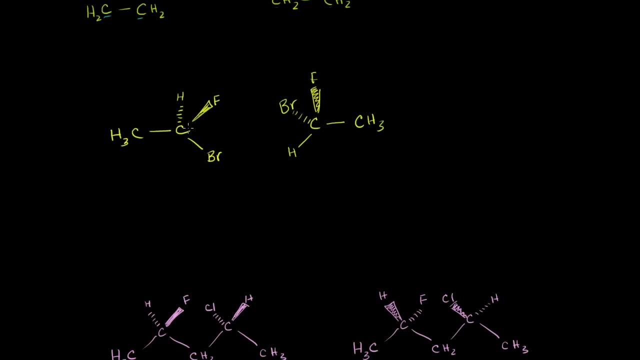 It is an asymmetric carbon. It is bonded to four different groups: fluorine, bromine, hydrogen and then a methyl group, And so is this one, And they're both made up of the same things. You have the carbon, and not only are they. 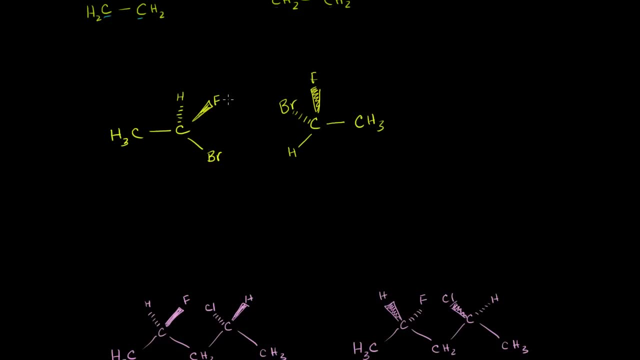 made up of the same things, but the bonding is the same. So carbon to a fluorine, carbon to a fluorine, carbon to a bromine, carbon to bromine, Carbon to hydrogen in both, and then carbon to the methyl group in both. 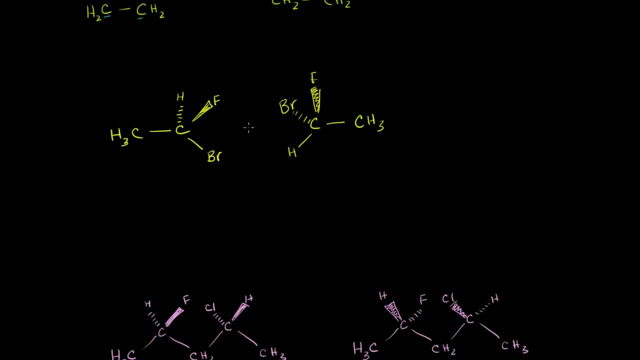 But they don't look quite the same. Are they mirror images? Well, no, This guy's mirror image would have the fluorine popping out here, the hydrogen going back here, and then would have the bromine pointing out here. Let's see if I can somehow get from this guy to that guy. 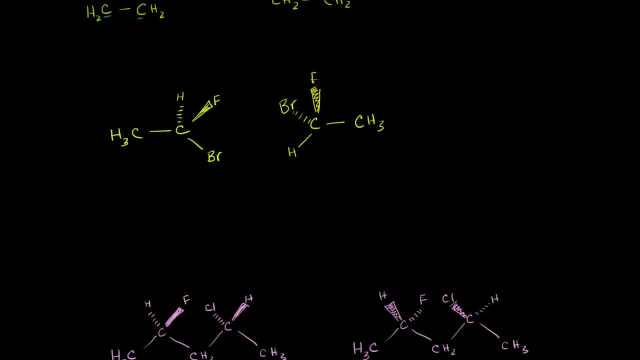 Let me flip this guy first. A good thing to do would be to just flip. Let me see the fastest way I could potentially get there. Well, let me just flip it like this. So I'm going to flip out of the page. you can imagine. 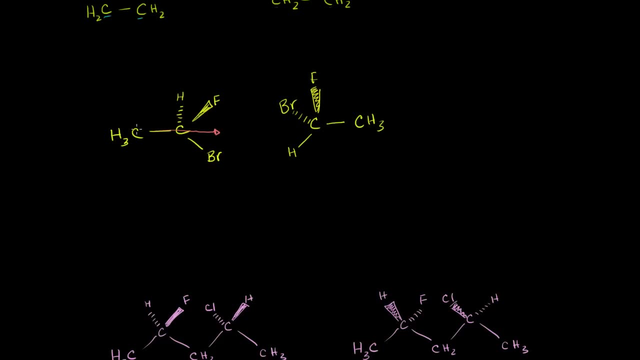 I'm going to flip it like this. So I'm going to take this methyl group and then put it on the right-hand side And you can imagine I'm going to turn it so it would come out of the page and then go back down. 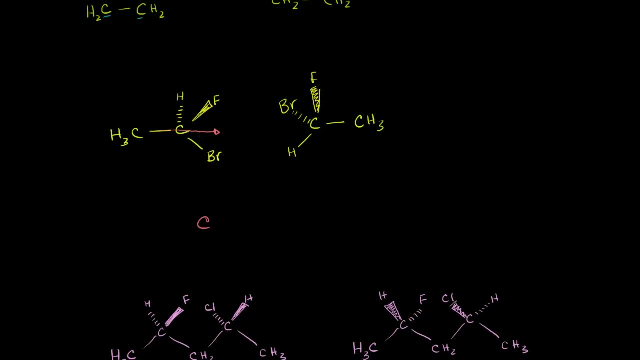 So if I did that, what would it look like? I would have the carbon, this carbon, here, I would have the methyl group on that side, And then, since I flipped it over, the bromine was in the plane of the page. 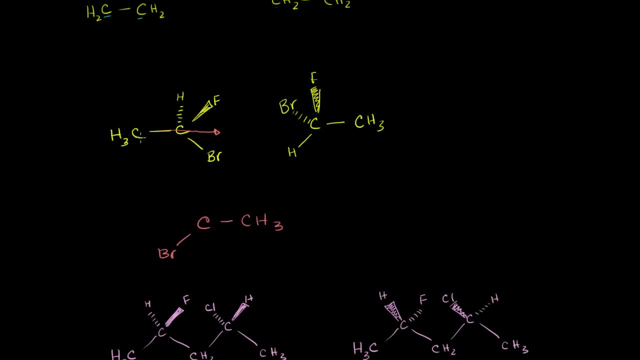 It'll still be in the plane of the page, But since I flipped it over, the hydrogen, which was in the back, will now be in the front and the fluorine will now be in the back, because I flipped it over. 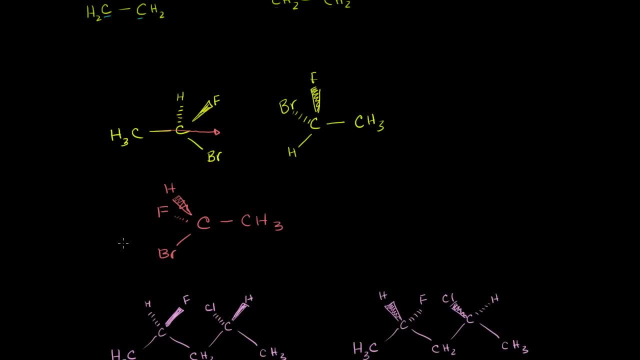 So the fluorine is now in the back. Now, how does this compare to that? Let's see if I can somehow get there. Well, if I take this fluorine and I rotate it to where the hydrogen is, and I take the hydrogen and rotate it to. 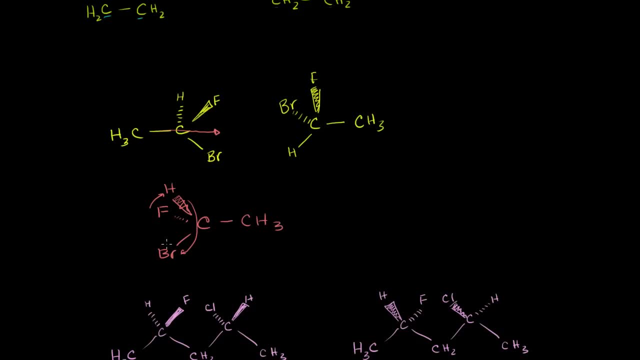 where that's all going to happen at once, to where the bromine is, and I take the bromine and rotate it to where the fluorine is. I get that, So I can flip it and then I can rotate it around this bond. 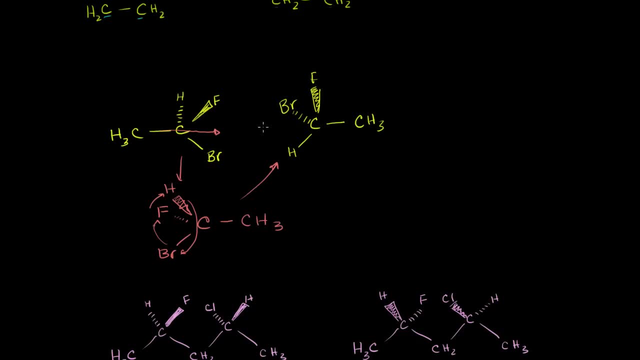 axis right there and I would get to that molecule there. So even though they look pretty different, with a flip and a rotation, you actually see that these are the same molecule. Next one: So let's see what do we have here? 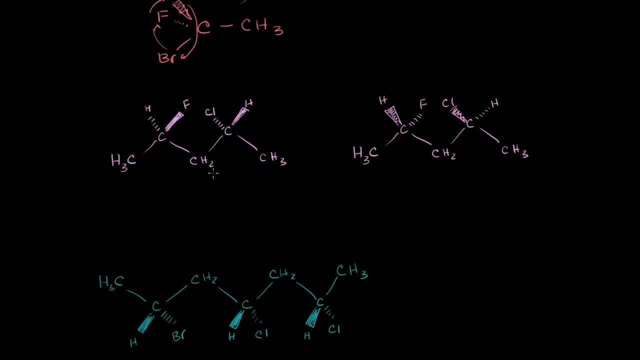 Let me switch colors. So over here, this part of both of these molecules look the same. We have the carbons on both of them. This carbon looks like a chiral center. It's bonded to one, two, three different groups. 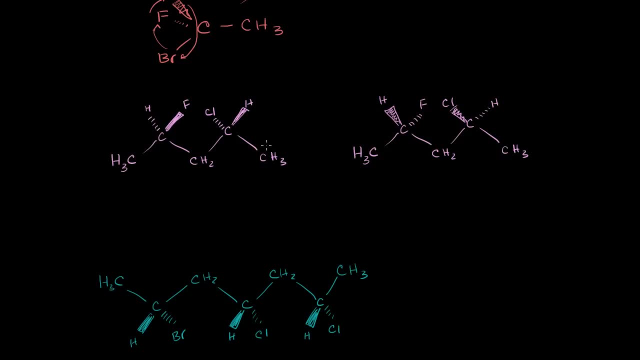 You might say: oh, it's two carbons, but this is a methyl group, and then this side has all this business over it. So this is definitely a chiral carbon. And over here, same thing: It's a chiral carbon. 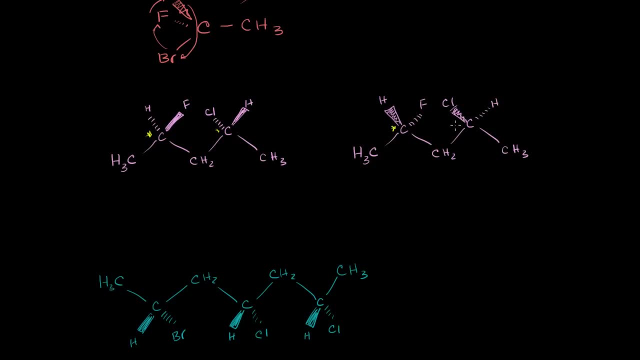 And this has the same thing. It's bonded to four different things. So each of these molecules have two chiral carbons, and it looks like they're made up of the same things. And not only are they made up of the same things, but the 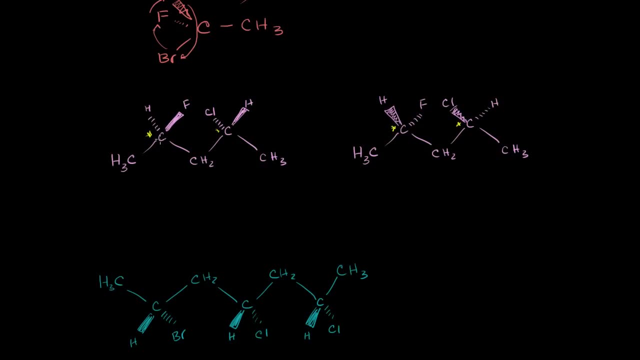 bonds are made in the same way, So this carbon is bonded to a hydrogen and a fluorine, and then two other carbons- same thing- a hydrogen and a fluorine carbon. it looks like it's bonded to a hydrogen and a chlorine. 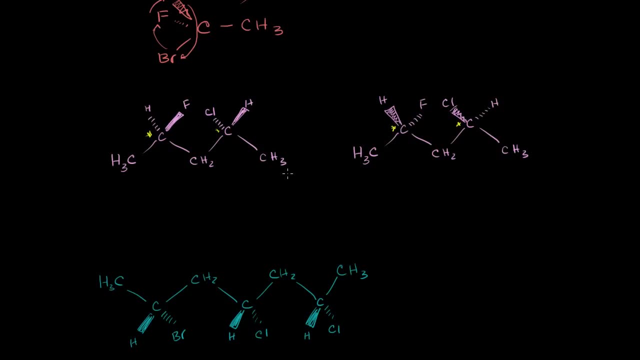 So it's made up of the same constituents and they're bonded in the same way. So these look like, but the bonding is a little bit different. Over here, on this one on the left, the hydrogen goes in the back, and over here the hydrogen's in the front. 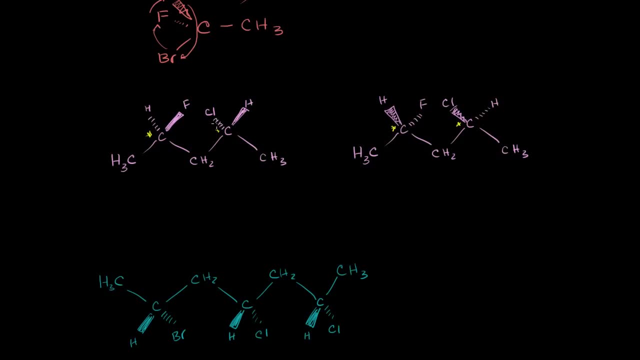 And over here the chlorine's in back and over here the chlorine's in front. So these look like stereoisomers You saw earlier in this video. you saw structural isomers. they're made up of the same things, but the connections 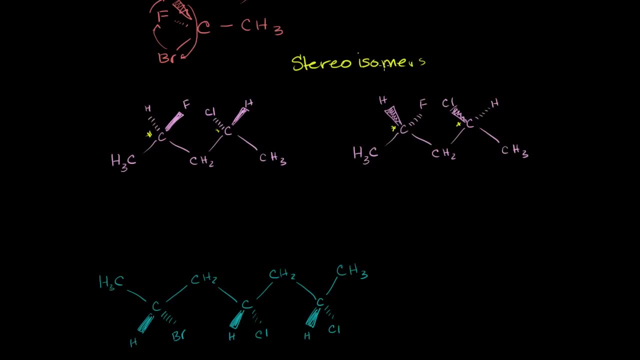 are all different Stereoisomers. they're made up of the same thing, the connections are the same, but their three-dimensional configuration is a little bit different. For example, here on this carbon, it's connected to the same things as this carbon, but over here, the fluorine's. 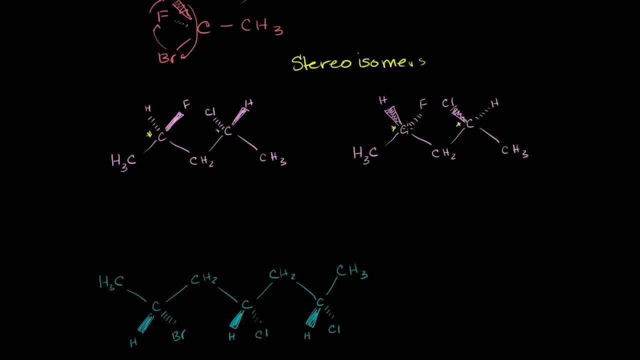 out front and over here the fluorine's out front, over here the fluorine's backwards. And the same thing for the chlorine here. It's back here and it's front here. Now let's see if they're related. I guess in a more. 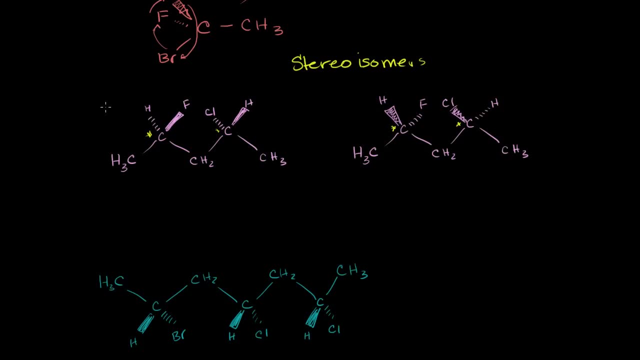 nuanced way. Well, you could imagine putting a mirror behind this molecule. If you put a mirror behind this molecule, what would its reflection look like? So if you put a mirror behind it, in the image of the mirror, this hydrogen would now, since the mirror's behind. 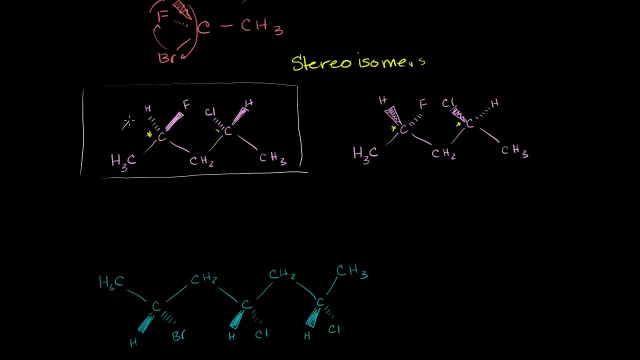 this whole molecule, this hydrogen's actually closer to the mirror. So in the mirror image you would have a hydrogen that's pointed out, and then you would have the carbon and then you would have the fluorine being further away. And same thing in the mirror image here you would have the 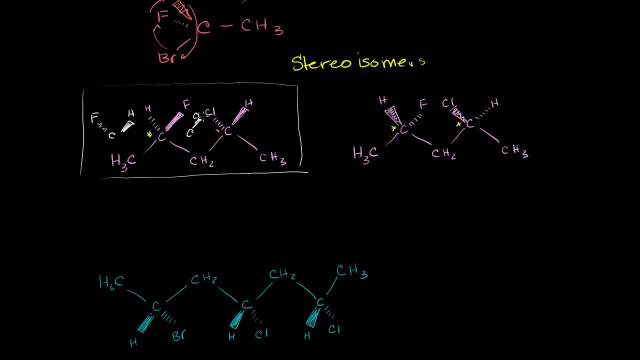 chlorine coming closer, since this chlorine is further back, closer to the mirror, and then you would have the hydrogen pointing outwards, like that, And then obviously the rest of the molecule would look exactly the same. And so this mirror image that I just thought about in white is: 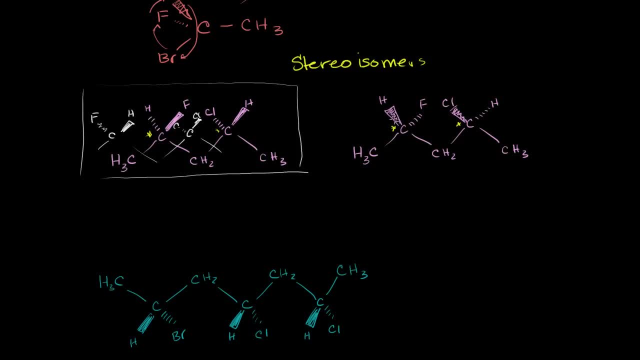 exactly what this molecule is. Hydrogen pointing out in front. hydrogen pointing out in front. You know you might say: wait, this hydrogen is on the right, this one's on the left, It doesn't matter. This is actually saying that the hydrogen's pointing out. 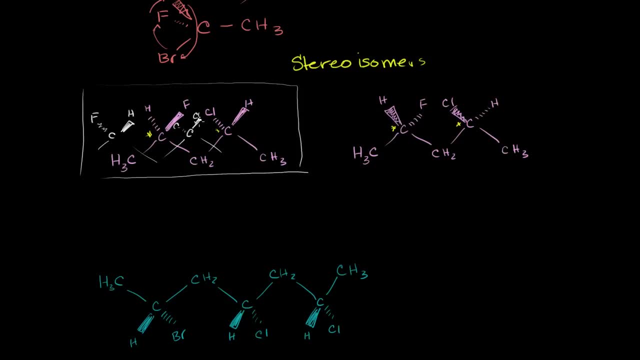 front fluorine's pointing out: back hydrogen out front fluorine, back chlorine out front hydrogen back chlorine out front hydrogen back. So these are actually mirror images, but they're not the easy mirror images that we've done in the past, where the 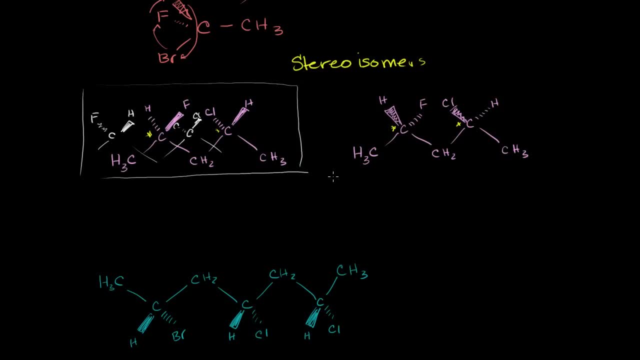 mirror was just like that in between the two. This one is a mirror image, where you'd place the mirror either on top of or behind one of the molecules. So this is a class of stereoisomers, and we've brought up this word before. 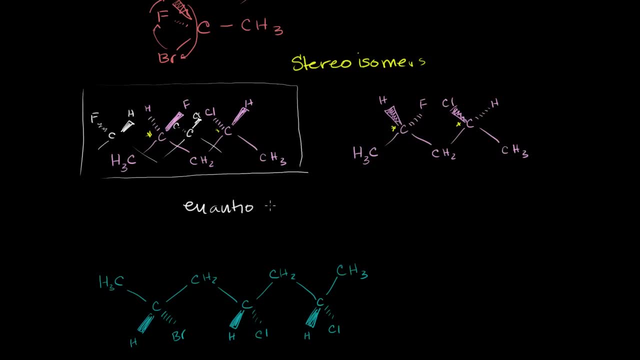 We call this enantiomers. So each of these are an enantiomer. I'll say they are enantiomers of each other. They're stereoisomers. They're made up of the same molecules, so they have the same constituents. 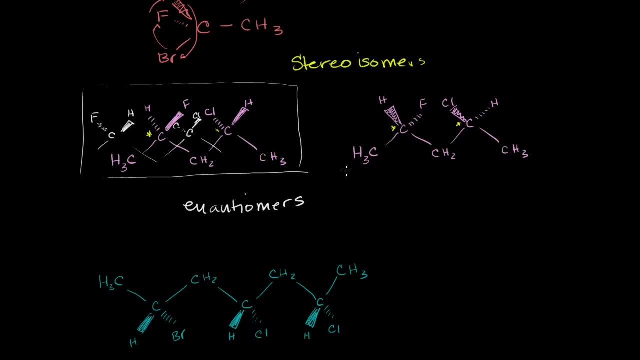 They also have the same connections. And not only do they have the same connections- that so far gets us a stereoisomer- but they're a special kind of stereoisomer called an enantiomer, where they are actual mirror images of each other. 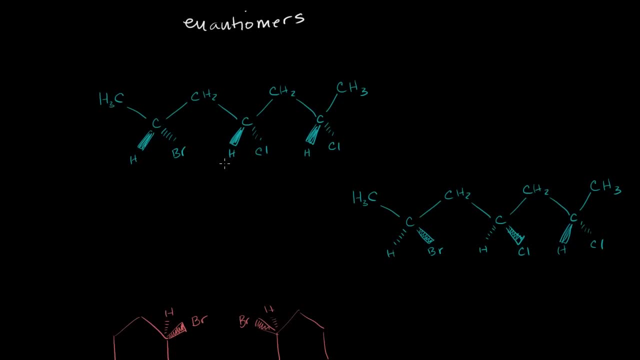 Now, what is this one over here in blue? Just like the last one, it looks like it's made up of the same things. You have these carbons, these carbons, these carbons and hydrogens up there. Same thing over there. 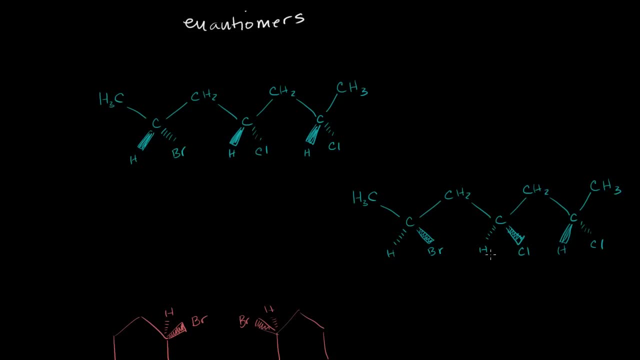 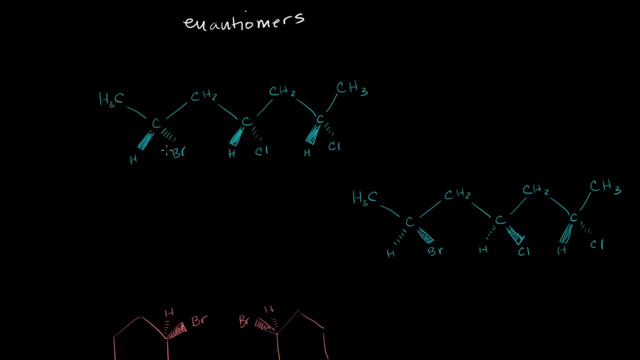 Well, let's make sure they're not the same molecule. first, Here, hydrogen's in the first, Here hydrogen's in the front. There, hydrogen's in the back. Here, hydrogen is in the back, Here hydrogen's in the front. 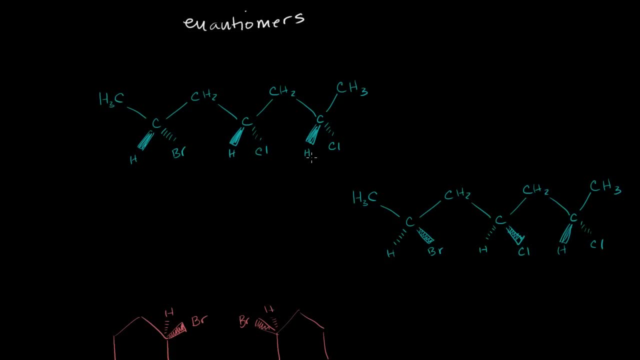 So they're not the same molecule. They have a different three-dimensional configuration, although the bond connections are the same. So these are stereoisomers. Let's see if they're enantiomers. So if we look at it like this, you put a mirror here, you. 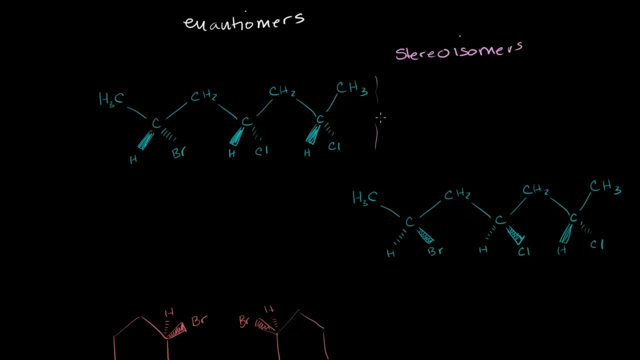 wouldn't get this guy over here. Then you would have a chlorine out front and a hydrogen. So you won't get it if you get a mirror over there. But if we do the same exercise that we did in the last pair, if you put a mirror behind this guy- and I'm just going to 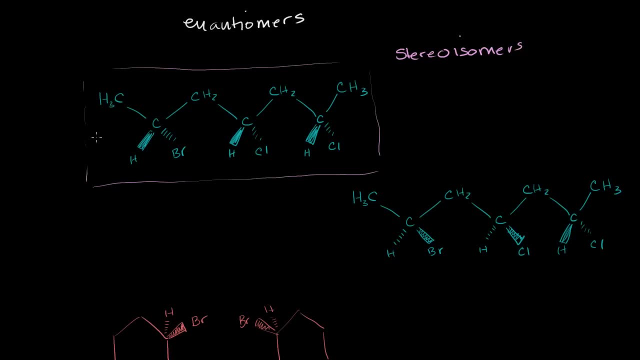 focus the stuff. that's just forward and back, because that's what's relevant if the mirror is sitting behind the molecule. So if the mirror is sitting behind the molecule, this bromine is actually closer to the mirror than that hydrogen, So the bromine will now be out front. 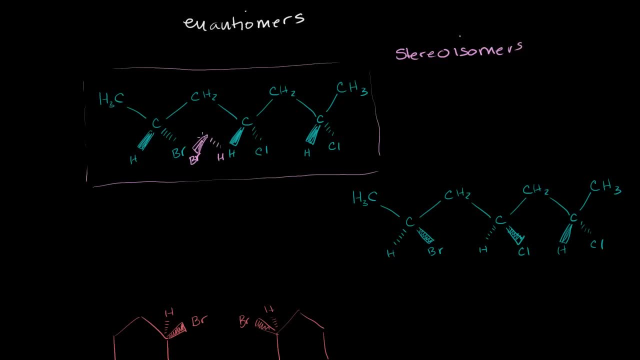 And then the hydrogen will be in back. This hydrogen will be in the back. I'm trying to do kind of a mirror image, if it's hard to conceptualize, and then that would all look the same, And then this chlorine will now be out front. 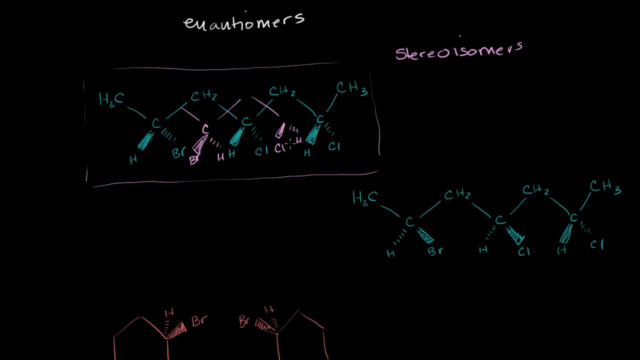 And this hydrogen will now be in the back in our mirror image, if we can visualize it, And then we have another one, And then this chlorine is closer to the mirror, that's kind of sitting on top of So in the mirror image. it would be pointing out. 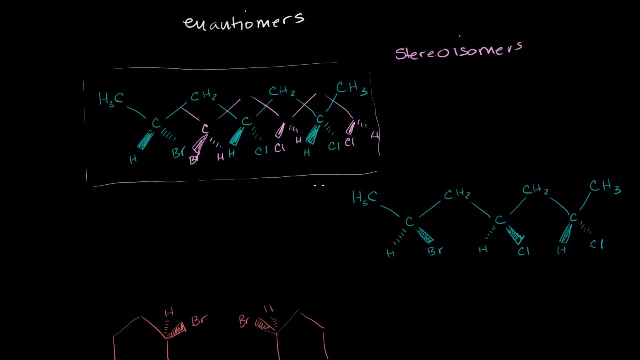 And then this hydrogen would be pointing back. Now let's see. Is our mirror image the same as this? So in the mirror image our bromine is pointing in the front, hydrogen in the back there. Then in our mirror image we have the hydrogen in the back. 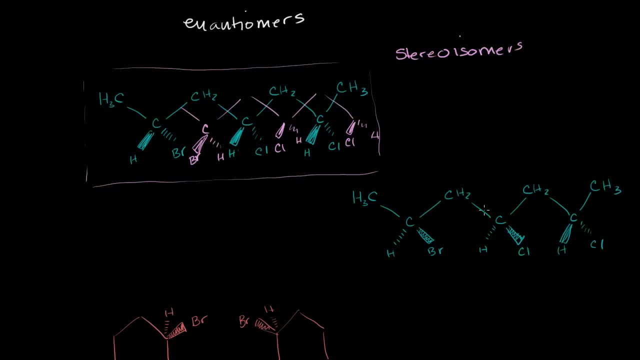 chlorine in front, Same there. So so far it's looking like a mirror image. And then in this last carbon over here, chlorine in front, hydrogen in back. But here we have chlorine in the back, hydrogen in front. So this part you could think of it this way: 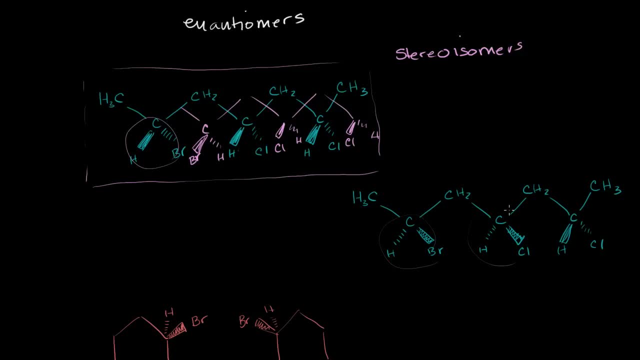 This is the mirror image of this. This is the mirror image of this part, But this is not the mirror image of that part. So, when you have a stereoisomer that is not a mirror, when you have two stereoisomers that aren't mirror images of each, 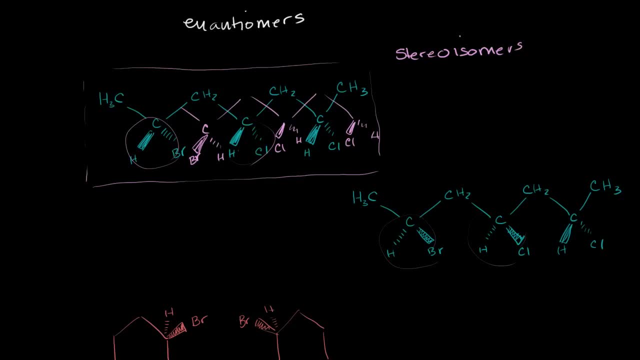 other. we call them diastereomer. I always have trouble saying that. Let me write it: These are diastereomers, which is essentially saying it's a stereoisomer, that is not an enantiomer. What does it mean? 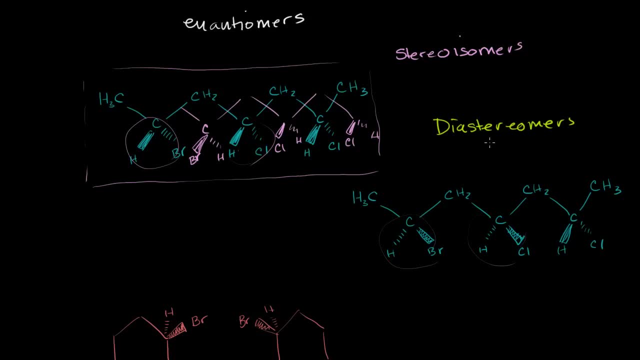 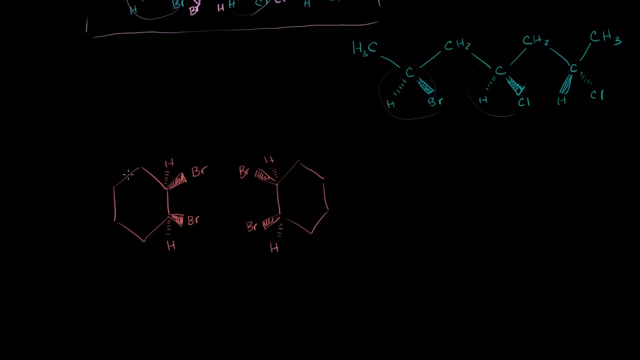 Stereoisomer, not an enantiomer. A stereoisomer is either going to be an enantiomer or a diastereomer. Now let's do this last one. Let's see, We have this kind of cyclohexane ring. 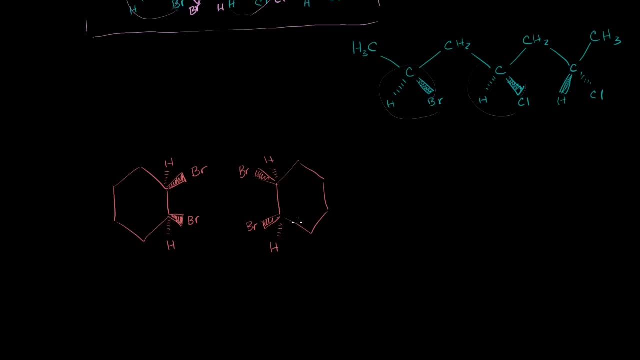 And they have a bromo on, I guess, the number one and the number two group. depending on how you think about it, It looks like they are mirror images of each other. We could put a mirror right there And definitely they look like mirror images. 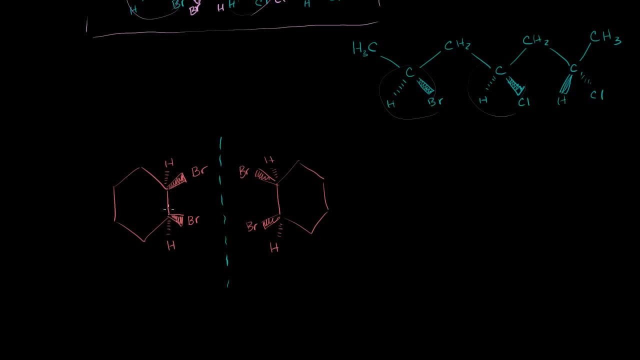 And this is a chiral carbon. here It's bonded to one carbon group. that is different than this carbon group. This carbon group has a bromine. This carbon group just has a bunch of hydrogens on it, if you kind of go in that direction. 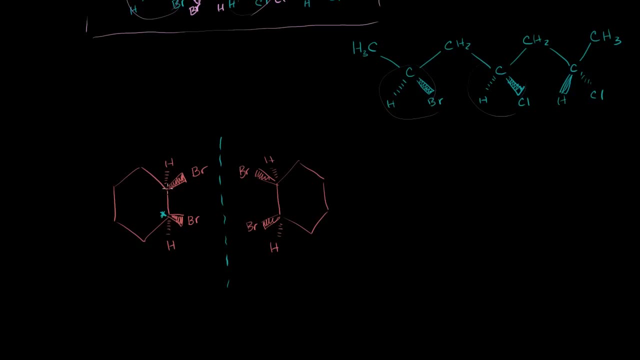 And it has hydrogen and then a bromine. So that is chiral. And then same argument: that is also chiral. And obviously this one is chiral and that is chiral, But if you think about it, they are mirror images of each. 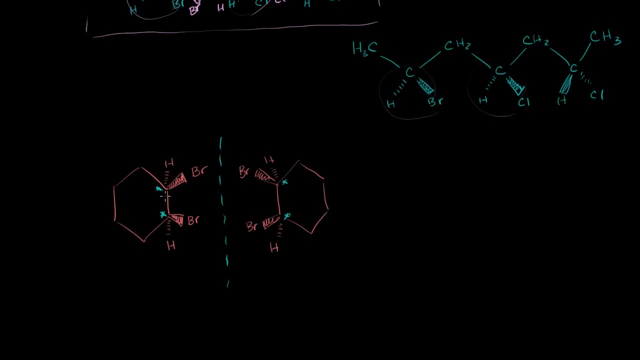 other and they each have two chiral centers or two chiral carbons. But if you think about it, all you have to do is flip this guy over And you will get this molecule. These are the same molecules, So it is the same molecule.